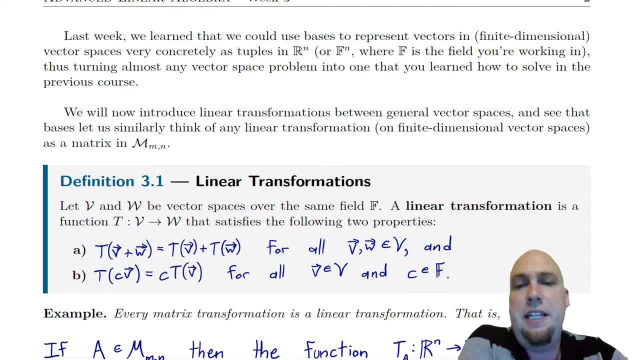 but it could be different And it's got to have two properties for it to actually be a linear transformation rather than just any old function. The first property is: if you sum up two vectors and then apply the linear transformation, you're going to have a function. that's going to be. 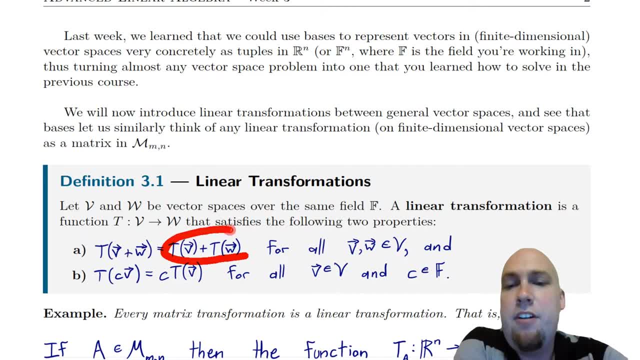 the function, You get the same thing as if you apply that function and then add them up. In other words, it sort of behaves well with vector addition right, And the other property is sort of the same thing, except for scalar multiplication. If you multiply a vector by a scalar and then 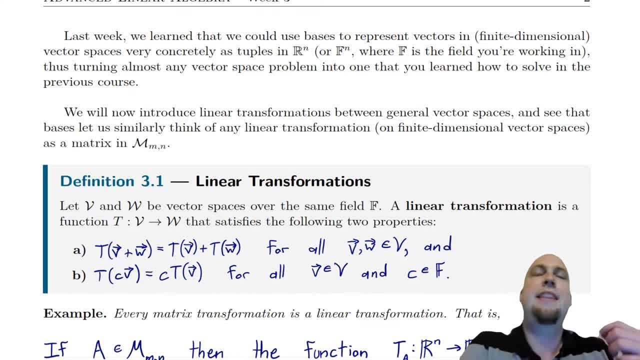 apply the function, you get the same thing as if you apply the function and then multiply by the scalar. Okay, so that's maybe a little bit abstract and you know, still seems like why those two properties? but let's go through sort of the motivating example here. Let's see why linear. 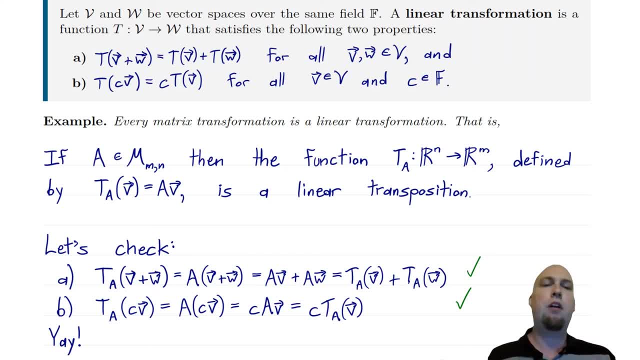 transformations are really a generalization, something that you've already seen before in introductory linear algebra, And the generalization, the thing that you've already seen in introductory linear transformation, is matrices. Like linear transformations are just the generalization of matrices, And here's how that works. Suppose that you've got some matrix: Here it's an m by n. 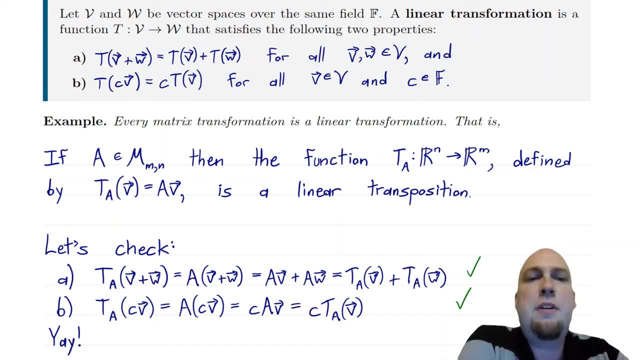 matrix. What you can do is, once you're given that matrix, you can define a function between two vector spaces, And this time the vector spaces are Rn and Rm. We can think of that matrix as sending n-dimensional vectors to m-dimensional vectors. in this way, You define some function. 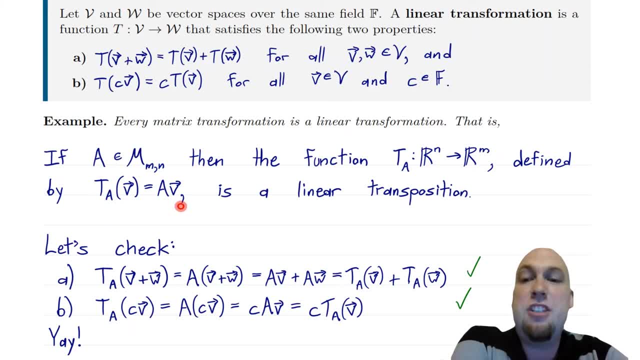 that we're going to call Ta, And the way that it works on vectors is it just multiplies that vector by the matrix And because of the size of the matrix here it sends n-dimensional vectors to m-dimensional vectors And it turns out that this is a linear transformation, This function. 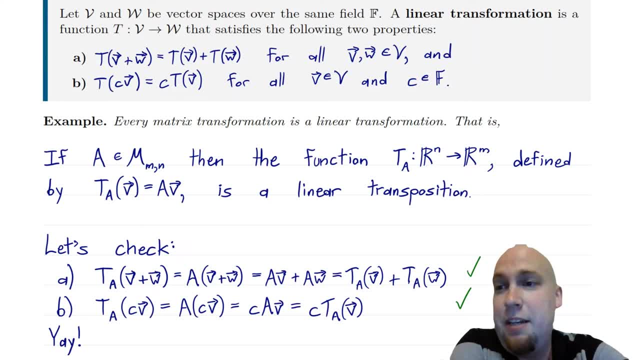 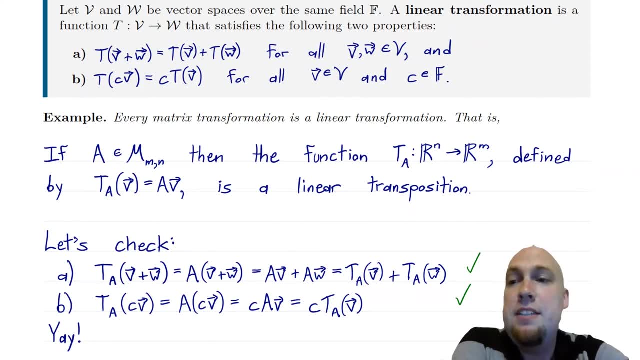 here is a linear transformation. Sorry for the typo here. That'll be corrected in the uploaded notes. So it's a linear transformation. And the way that you check that is you just check the two defining properties of linear transformations. You check these properties a and b up here. So let's do that, And to do that we just use properties. 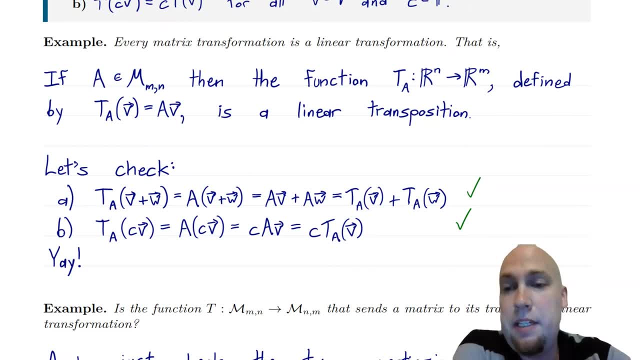 of matrices that we already know from the previous course. So the first property that we want to check is: we want to see that, hey, if we're applying this function here to the sum of two vectors, I'd better get the same thing as if I apply that function to one vector plus that. 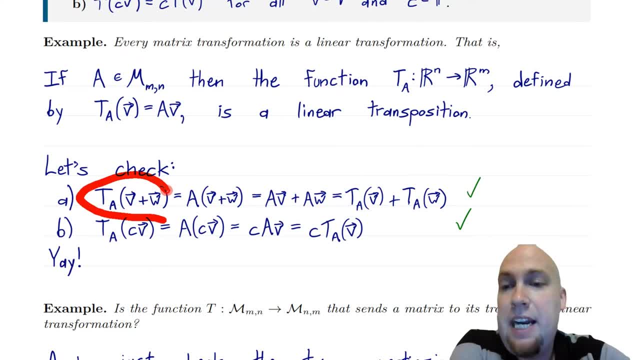 function applied to the other vector. So how's that? How's that work? Well, by definition, this function applied to v plus w is just a times v plus w. All right, And one of the properties of matrices that we know is that a times v plus w is a times. 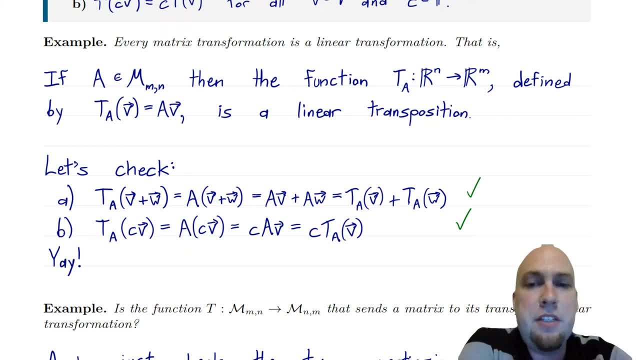 v plus a times w. We call that distributivity in the previous course because it's sort of multiplication, distributing over addition. OK, And then a times v, well, that's just ta of v, And a times w that's just ta of w. We're just using the definition of this function from back. 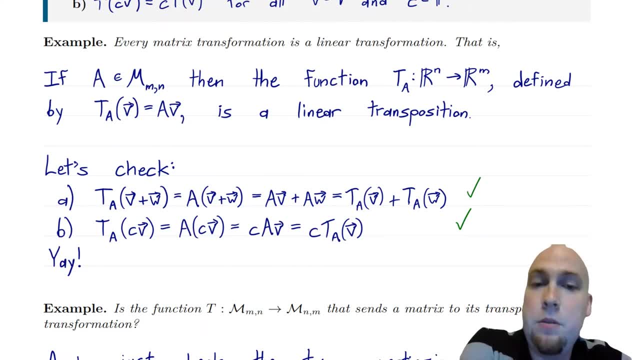 here. OK, And that's exactly what we want. So, yay, property a, Property a holds Property b is almost identical, right? It's just hey, what is this function applied to c times v? Well, it's just a times c times v, And then again, property is a matrix. 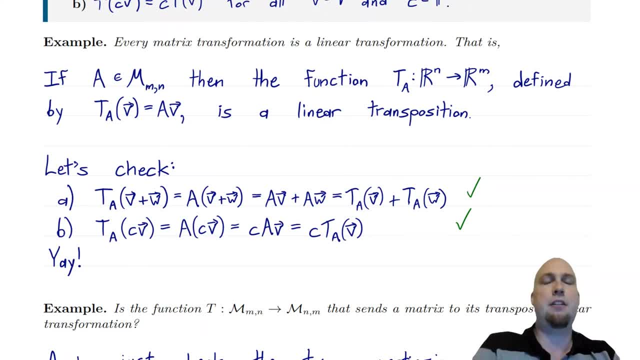 multiplication. I can pull that scalar c out in front. It doesn't matter if I do matrix times scalar times vector or scalar times matrix times vector. You get the same thing either way. So this is the same as c times a times v, which is c times ta of v. right av, here is ta of v. 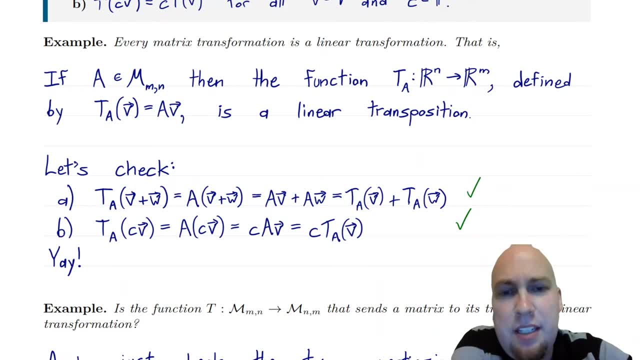 All right, So that's all that we needed to check. I mean, most of these equalities here are nothing more than changes of notation, really Like four of these equalities here are just making this substitution of notation. It's just function. 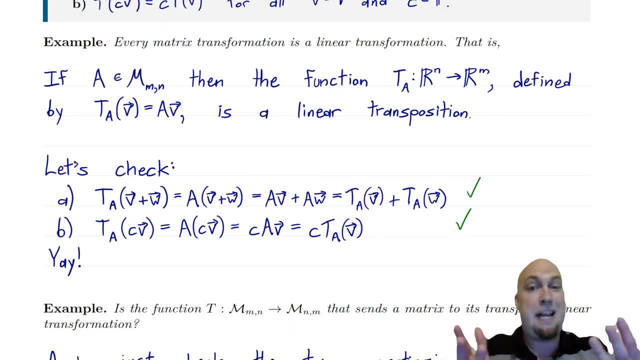 applied to vector is matrix times vector. There's actually not much math really going on there. These two central equalities are really the mathematical steps where something had to be shown, but we showed it in the previous course, All right. So yeah, matrices- matrices are linear. 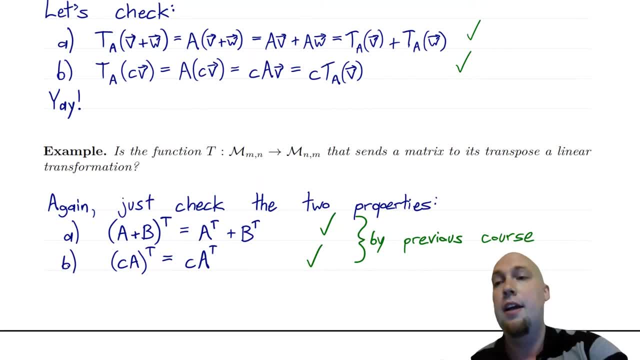 transformations. They're functions that act on vectors and they act sort of in a way that respects our vector space operations. But there are lots of other functions that act on vectors. There are other interesting linear transformations out there too. So, for example, is the function: 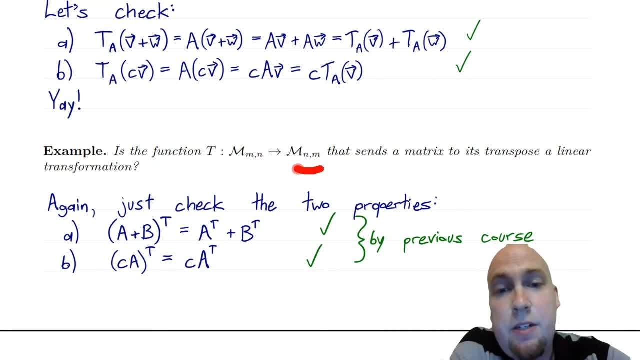 which takes an m by n matrix and spits out an n by m matrix. is the function that transposes a matrix. is that a linear transformation? Okay, And it's going to turn out that? yeah, it is Okay. So how? 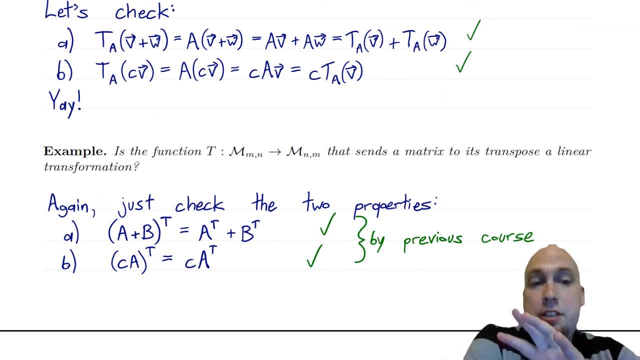 do we check this Again. you have two properties that you got to check. Okay, Linear transformations: they depend on two things. The first thing is: well, if I apply the linear transformation to the sum, do I get the same thing as if I apply the linear transformation to the sum? 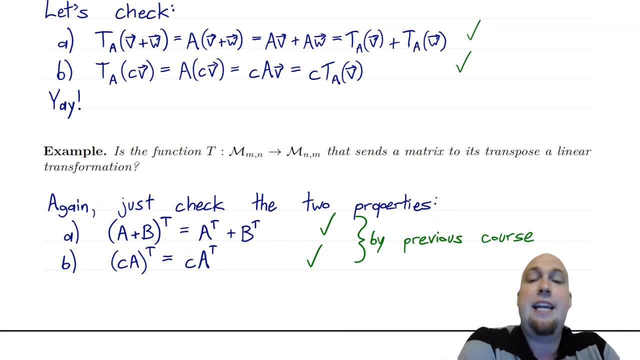 Do I get the same thing as if I apply the linear transformation to them individually and then add them up. In other words, in this case that means is A plus B transpose the same as A transpose plus B transpose. And yeah, it is Okay Again. you learned this in the previous course. Okay To. 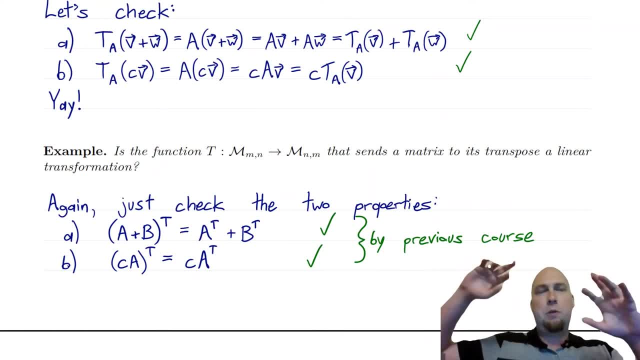 prove this property. you just work entry-wise right. Think about what the transpose does. All it does is sort of shift the positions of the entries in the matrix. Okay, So if you add them up and then shift the positions, you get the exact same thing as if you shift the positions of both. 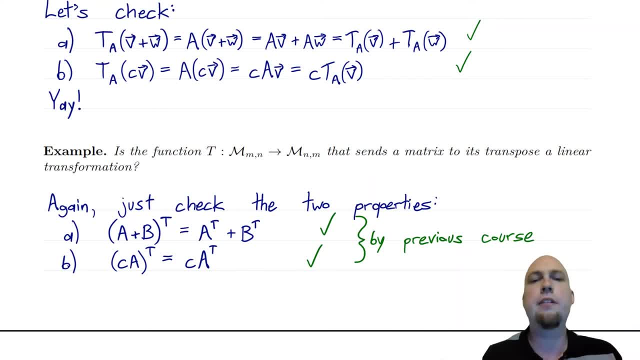 of them and add them up, because addition is just entry-wise. There's sort of nothing weird going on here. Okay, Property B is very similar. If you scale or multiply by C and then transpose, do you get the same thing as if you transpose and then scale or multiply by C? Yeah, you do. Okay. 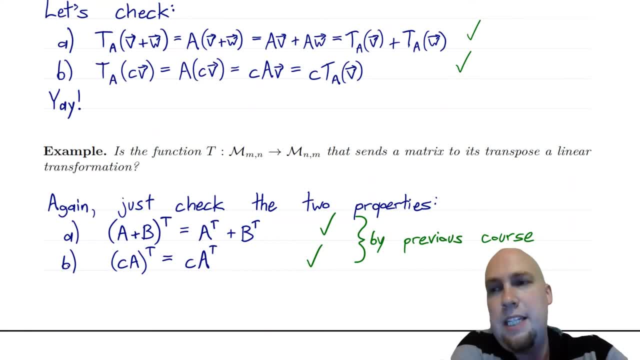 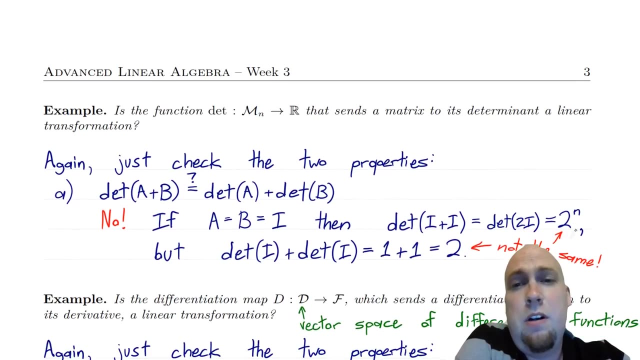 Just work entry-wise. You can work entry-wise and prove that straightforwardly Again. we saw that in the previous course. So the upshot is: yes, the transposition function, the function that spits out the transpose of a matrix, that is a linear transformation, All right, Well, if we go to. 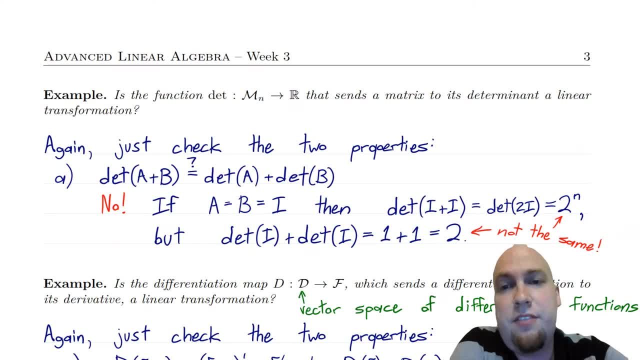 a slide. It's a slightly more exotic function. What about the determinant function? Okay, So if you've forgotten what the determinant is, I'll try to remind you of just the basics as we go through this. But the determinant, remember that's the function that it takes in a matrix. And then we 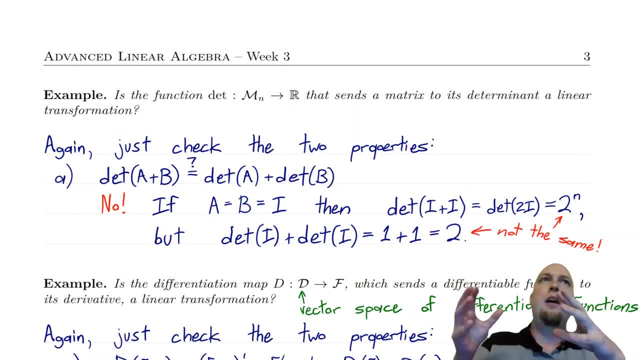 had these complicated ugly formulas for it. But what it showed you was- it told you- sort of the signed volume of that linear transformation of that matrix. It sort of told you, hey, if you feed the unit cube into this matrix, how big is it when it comes out? Okay, It's a measure of the size of 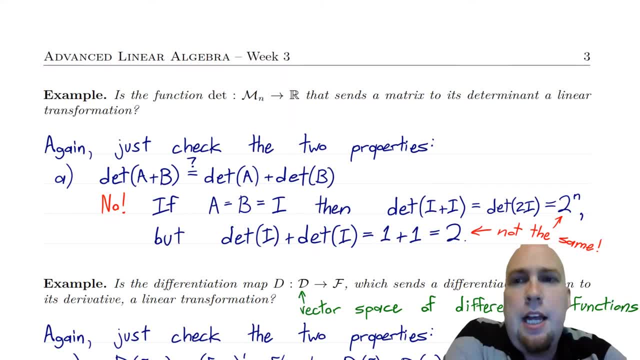 the matrix. basically, All right. So this function, the determinant, is that a linear transformation. Okay, So let's check it. Okay, So we got to check two properties again. Property A: Is it true that the determinants of A? 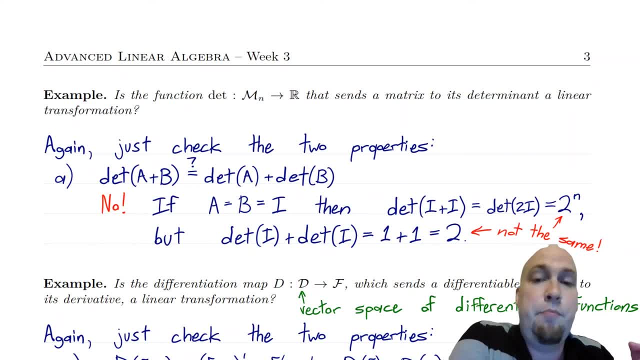 plus B equals the determinants of A plus the determinants of B. Okay, And you could spend all day trying to prove that. but maybe the fact that we did not see that as a property of the determinant back in linear algebra one, maybe that signals that there's something wrong here. 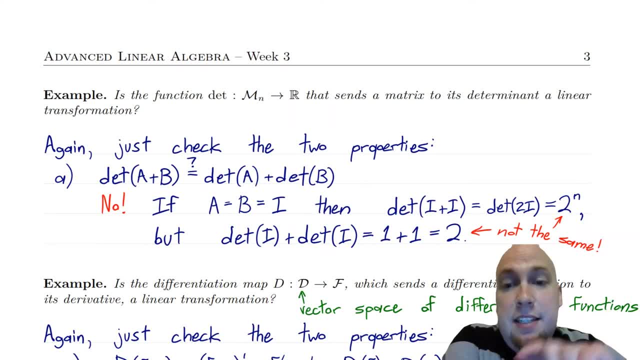 Okay, That property is not true. This property is not true. The determinant is not additive. Okay, And to show that it's not true, you just need a single counterexample. So here's one particularly nice counterexample. What if A and B are both the? 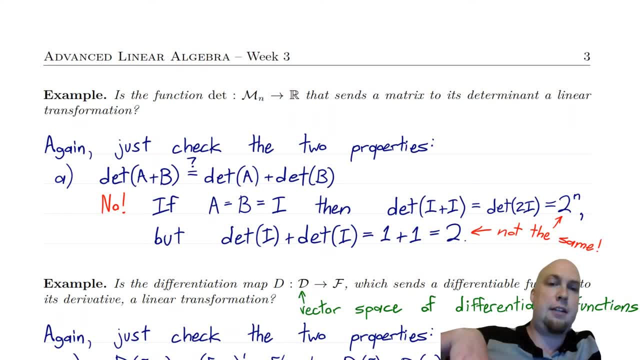 identity matrix. So it has ones on the diagonal and zeros off diagonal, All right. Well then, determinants of the sum of them is determinants of I plus I, which is determinants of 2I, And then again remember. so here we've got the determinants of the matrix that has twos on its diagonal, and 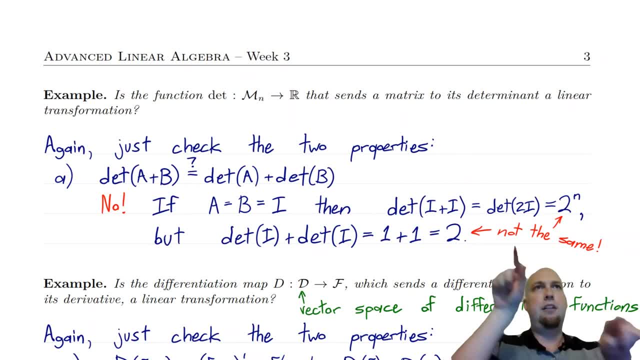 zeros elsewhere. And we had a theorem in the previous course that said if you have a diagonal matrix, or even more generally, if you have a diagonal matrix you have a determinants of the product of those diagonal entries. So here you've just got N twos going down that diagonal, So the 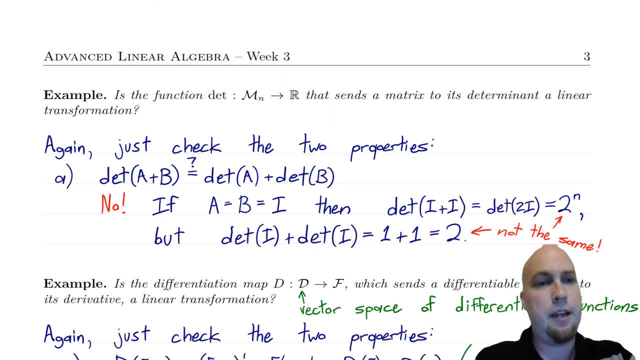 determinants is the product of all of them, which is two to the power N. All right, great. So that's what determinants of A plus B is. But on the other hand, the right-hand side is determinants of identity plus determinants of identity, And the identity matrices each have determinants equal to. 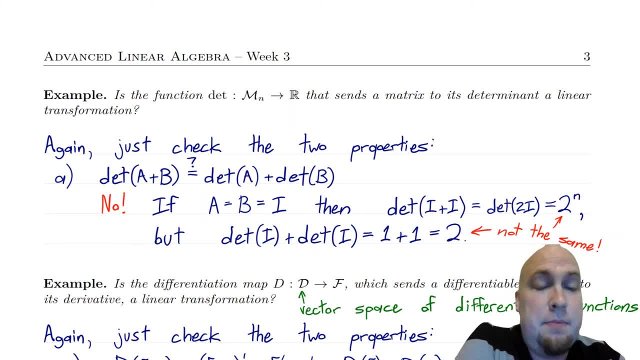 one. So you add them up, you just get two instead of two to the power N. So these quantities here are not the same. So this property fails. So it's not a linear transformation. Okay, and maybe two quick notes. I did not check property B anywhere, right, We only checked. 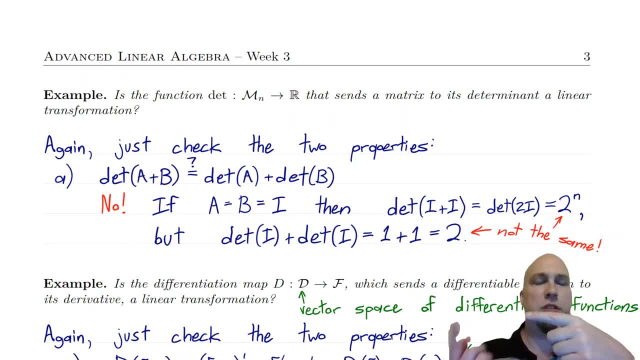 property A, And that's because we already showed the property A doesn't even hold. So we already know it can't be a linear transformation. As long as at least one of those two properties fails, it's not a linear transformation. So once one of them fails you don't need to check the other one. 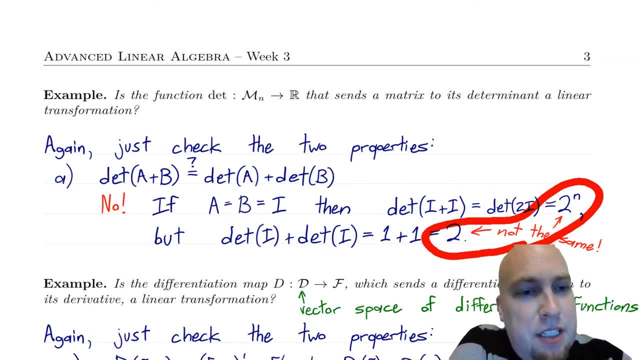 The other thing is: hey, we've got two and two to the power N. Well, there's one case where those properties fail, And that's when N equals one. And well, yeah, I mean, if the determinant of a one-by-one matrix is just that number itself, that is a linear transformation, The determinant on 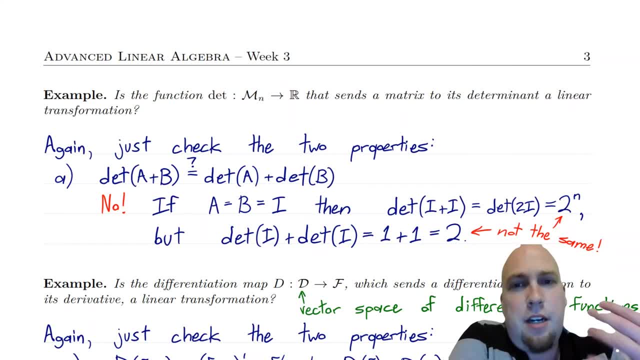 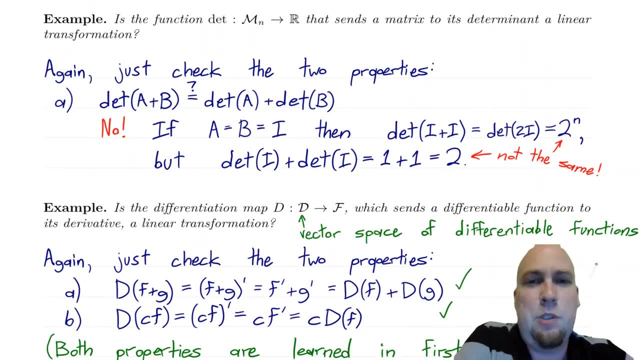 one-by-one matrices is just the identity function, So it's not a linear transformation for two-by-two or larger matrices, but it sort of trivially is for one-by-one matrices. We don't ever really consider one-by-one matrices anyway, We just call them scalars. Okay, so determinant, not a linear. 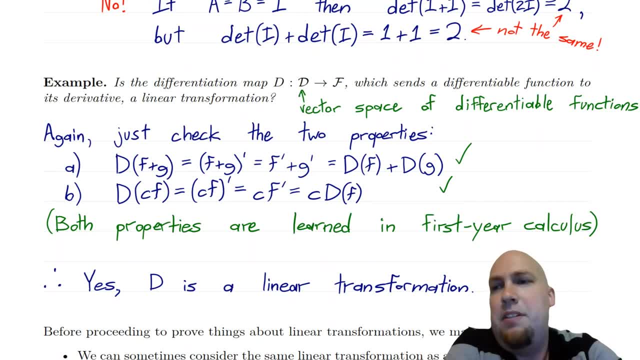 transformation. Let's go to one more kind of exotic example of something that is a linear transformation. So let's go to one more kind of exotic example of something that is a linear transformation. So is the differentiation map. so D, here is the function that takes the derivative. 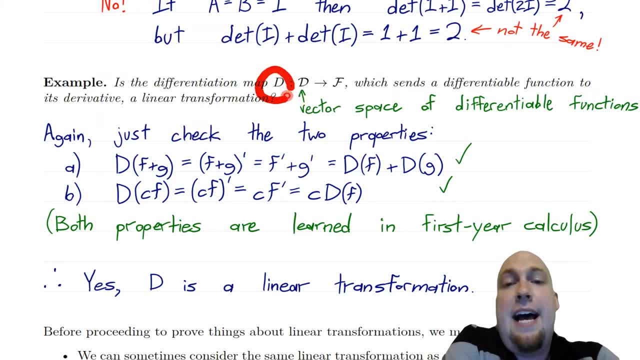 of a function. Okay, is that a linear transformation? Okay, and just a little note on the notation here, this curly D here. that's the vector space of all differentiable functions. It's the vector space of all functions that have a derivative. Okay, and then F, here is again just. 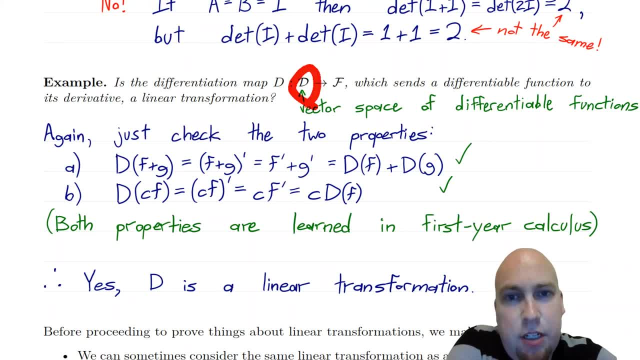 the vector space of all functions. All right. so D sends a differentiable function to just some function. All right, and this function acts by taking the derivative. Is that a linear transformation? So again we've got to check the two properties. Is the derivative of F plus G? 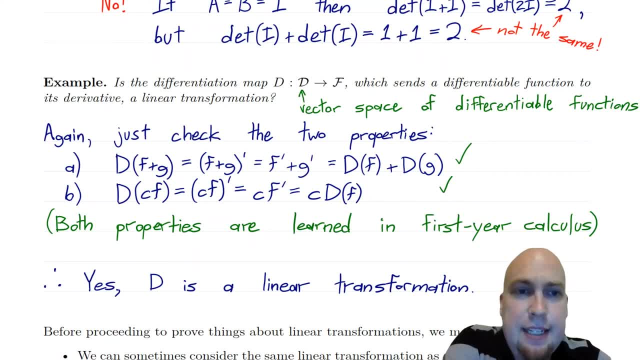 equal to the derivative of F plus the derivative of G. Yes, you learned that in first-year calculus. Is the derivative of scalar times F the same as scalar times, the derivative of F? Yes, you learned that in first-year calculus. Okay, and all of these intermediate steps are just converting. 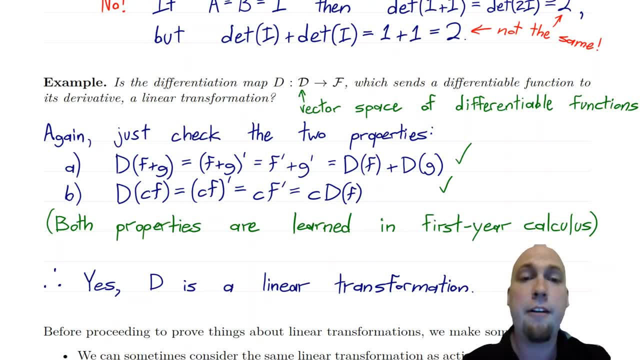 things back to notation that maybe you're a little bit more used to from first-year calculus. Okay, but yeah, so both of those properties hold and so, yeah, D is a linear transformation, The derivative is a linear transformation. All right, so that's really nice. That's going to be a nice example. 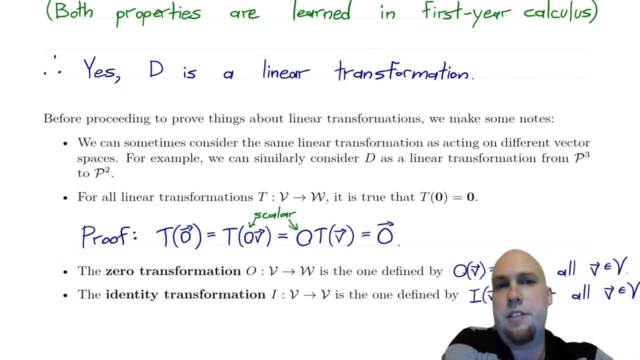 that's going to do some neat stuff as we go through the next week or two. All right, basically, what that's going to let us do is it's going to let us do linear algebra stuff to solve calculus problems. Okay, and before we finish off for today, just a couple of quick notes. So one thing to keep. 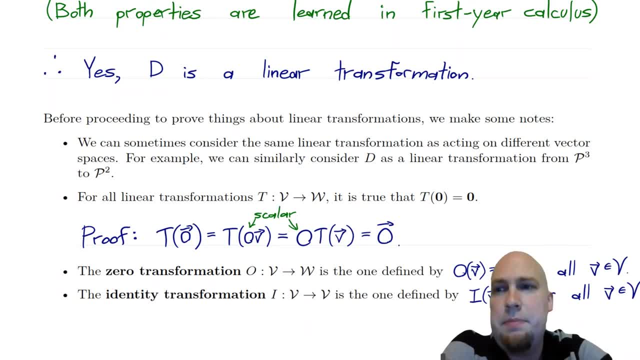 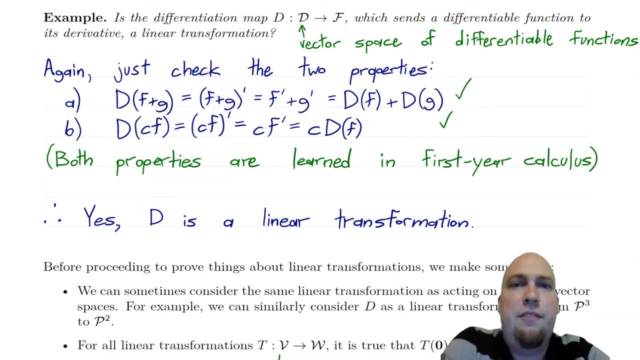 in mind is that linear transformations- they can act on multiple different vector spaces. Okay, so it depends a little bit on what vector spaces you're using. So here I said, you know, consider the derivative linear transformation acting on the vector space D and mapping into the vector space F. 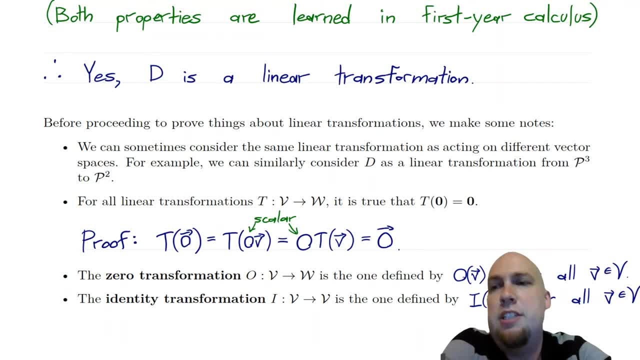 Well, I you know, I could also consider that linear transformation D that takes the derivative. I could consider it as acting on, say, P3 and mapping into P2,. right, Because if you take the derivative of a degree less than or equal to three polynomial, you get a degree. 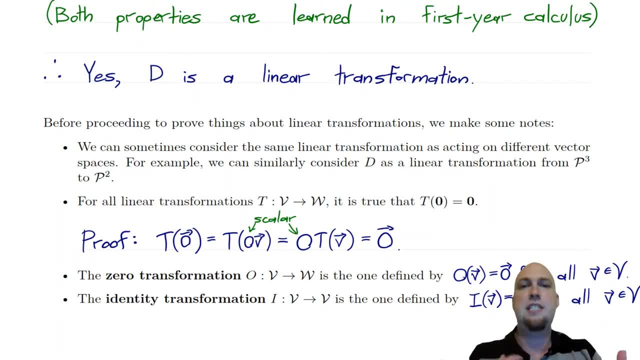 less than or equal to two polynomial, And that's okay too. So I can consider D acting on different vector spaces, depending on what my intention is with that linear transformation. All right, One other thing that's really useful to keep in mind. this really helps when checking that something is.